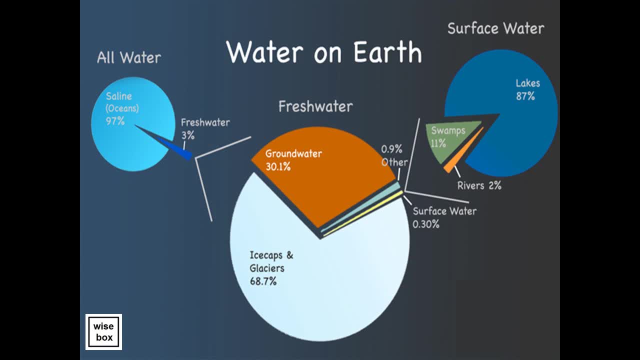 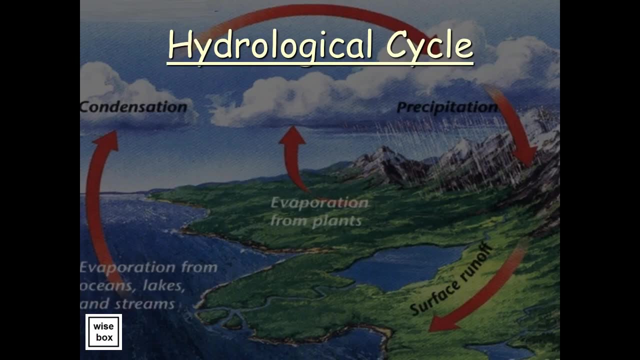 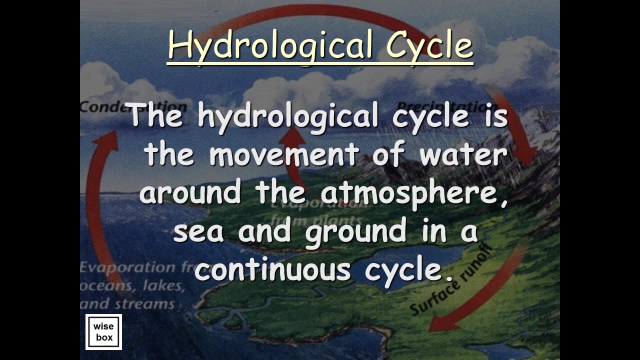 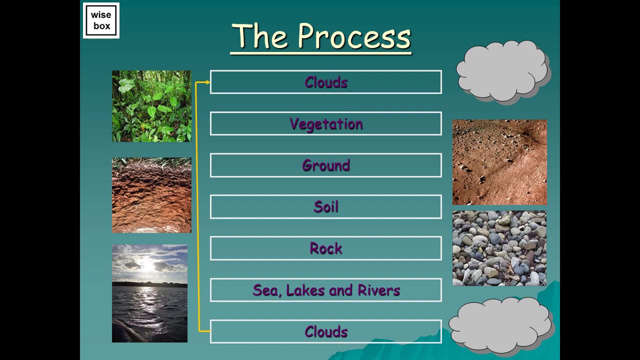 Such as saline water, fresh water and surface water. The hydrological cycle is the movement of water around the atmosphere, sea and ground in a continuous cycle. The process involves water going from the clouds to vegetation, ground, soil, rock. 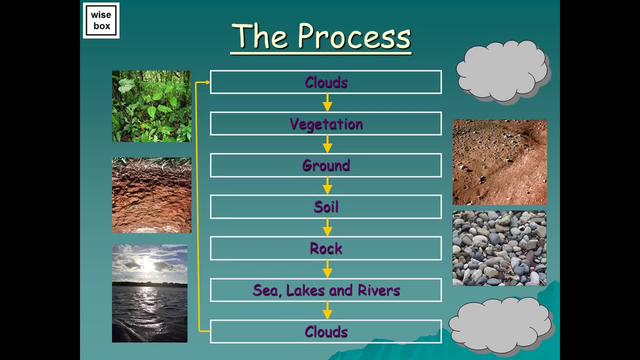 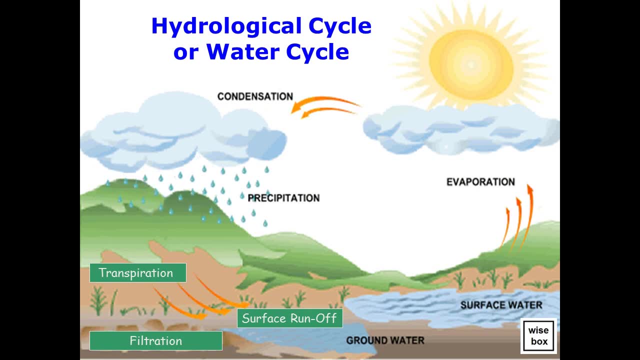 And back to the sea, lakes and rivers and back to the clouds. Here is an illustration of the hydrological cycle or the water cycle. It involves process such as evaporation, condensation, precipitation, surface runoff, subsurface runoff and transpiration. 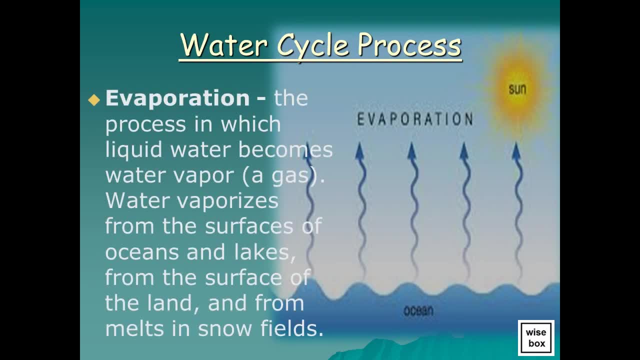 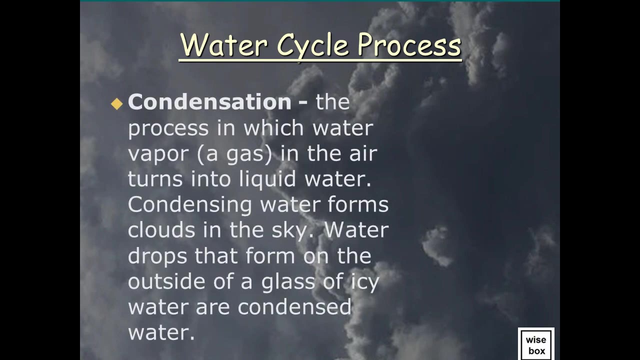 Evaporation is the process in which liquid water becomes water vapor, a gas. Water vaporizes from the surfaces of oceans and lakes, From the surface of the land and from melts in snow fields. Condensation is the process in which water vapor, a gas in the air, turns into liquid water. 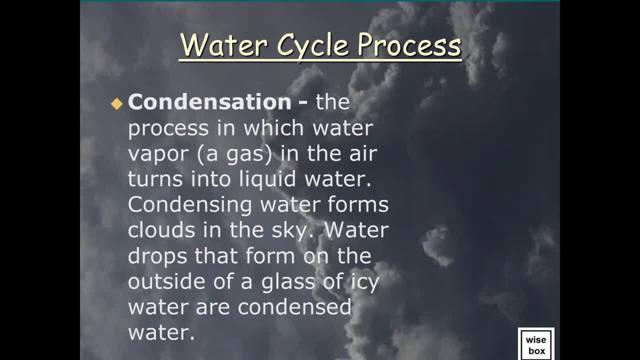 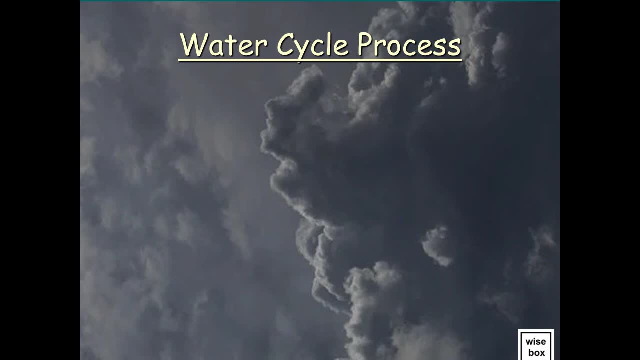 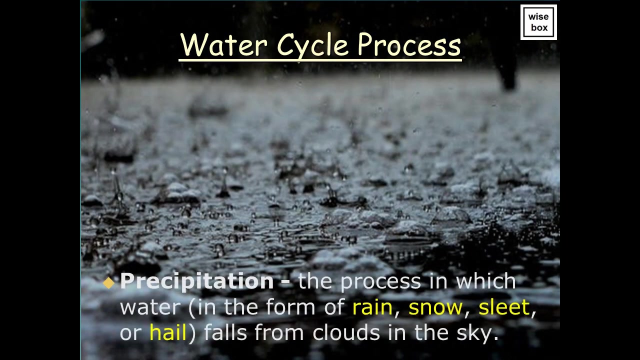 Condensing water forms clouds in the sky. Water drops that form on the outside of a glass of icy water or condensed water. Condensation is the process which creates clouds and so is necessary for rain and snow formation. Condensation is the process in which water in the form of rain, snow, sleet or hail falls from clouds in the sky. 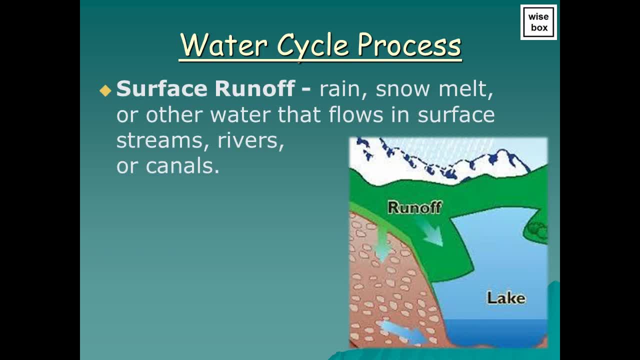 Surface runoff comes from rain, snowmelt or other forms of water that flows in surface streams, rivers or canals. Subsurface runoff comes from rain, snowmelt or other water that flows in underground streams, drains or sewers. 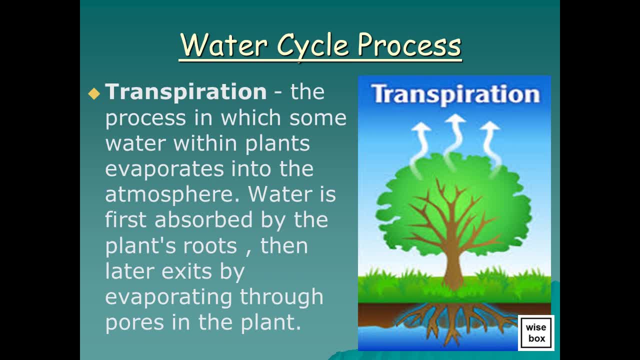 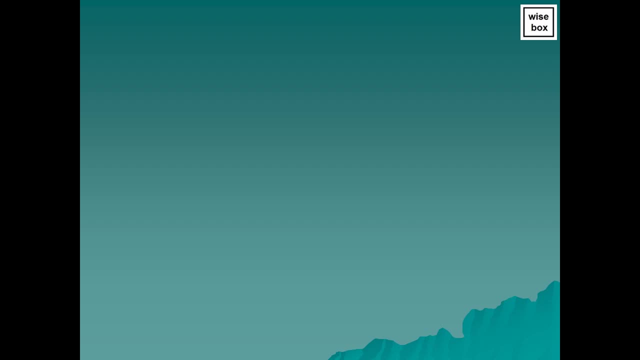 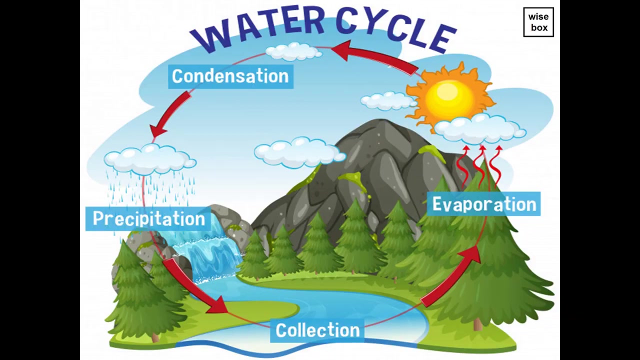 Transpiration is the process in which some water within plants evaporates into the atmosphere. Water is first absorbed by the plant's roots, then later exits by evaporating through pores in the plant. Here is an illustration of the hydrological cycle or the water cycle.